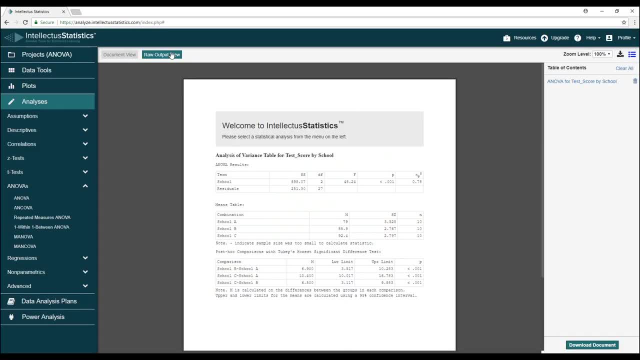 Here are the interpreted ANOVA results. Let's start with the raw output to see how we got here. At its most basic, the output of an ANOVA will consist of a single table, but it's common to see additional tables or plots. In this case you can see there's a table for descriptive statistics. 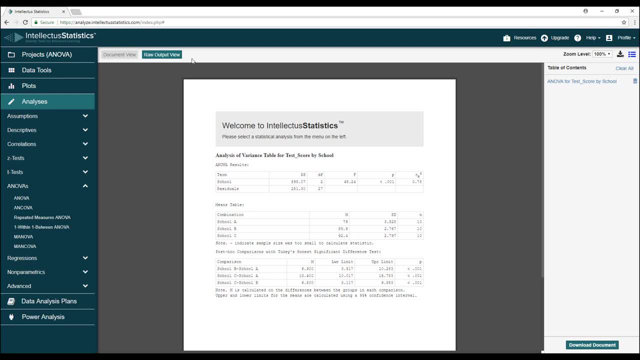 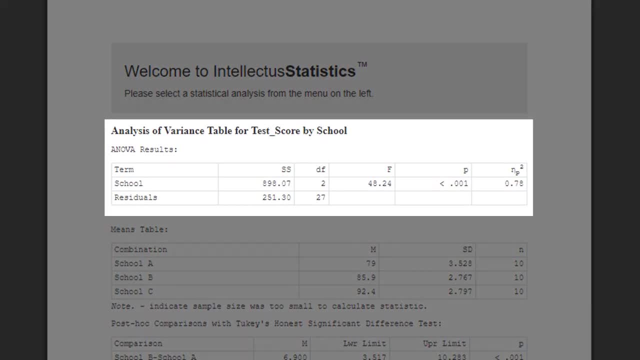 reporting the means and standard deviations of the groups and a table for post-hoc comparisons. For now, let's focus on the ANOVA table. The main ANOVA table contains information on the variance of the data and the sample size, as well as the results of the statistical hypothesis. 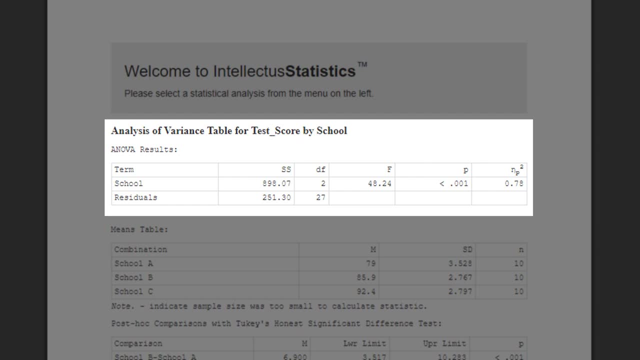 All the information in this table is useful for understanding the analysis at a deeper level, but at an initial glance, all you need to look at are these last two columns. The column labeled P is the probability value, or p-value. This number can be used to decide. 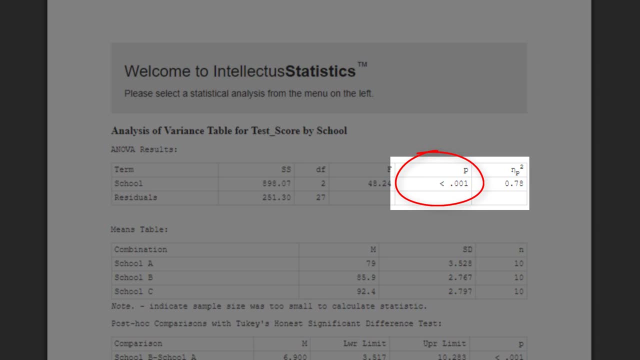 whether we call the result significant or not, This will always be a number between 0 and 1, and represents the likelihood of observing the result under the null hypothesis. In this example, p is less than 0.001.. This means, if we assume that the result is less than 0.001,. 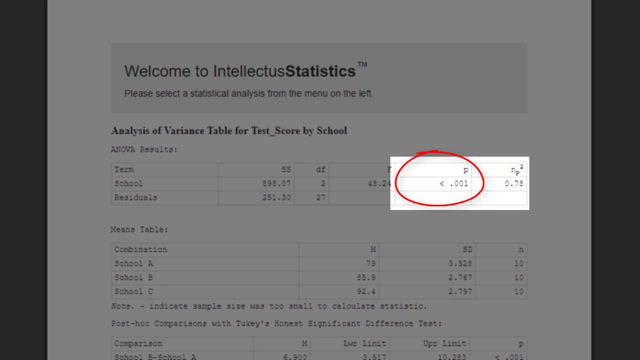 that there really is no difference in the students' test scores. there's less than a 1 in 1,000 chance that we would see a difference like this. It's still a possibility that these differences are just due to random chance, but it's very unlikely. That means we can say the result is statistically 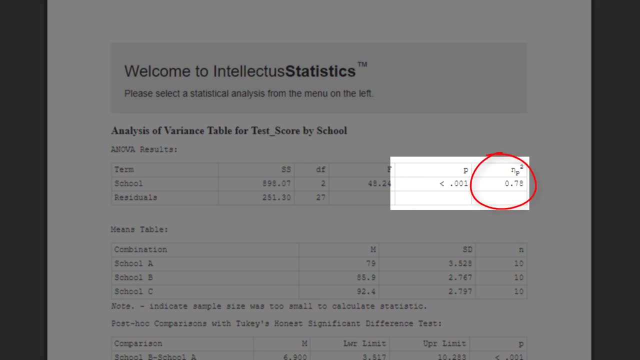 significant. Next, we need to look at the column labeled eta squared. This is called an effect size. statistic Effect sizes help put the result into context. P-values are a function of sample size. so if we're dealing with a very large sample size, say in the thousands or millions, 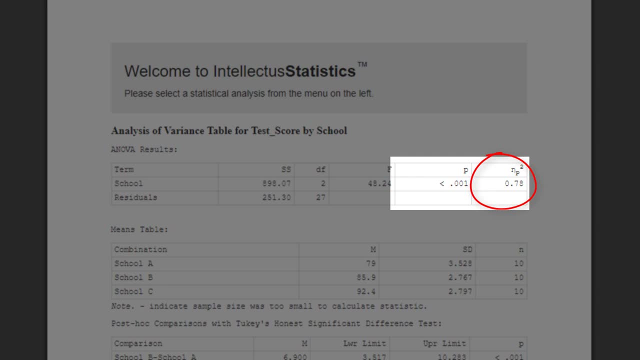 even a very tiny difference would be statistically significant. In the real world we probably don't care about these tiny differences, so effect size statistics give us a way to decide how we want to interpret the result. Like the p-value, eta squared is also a. 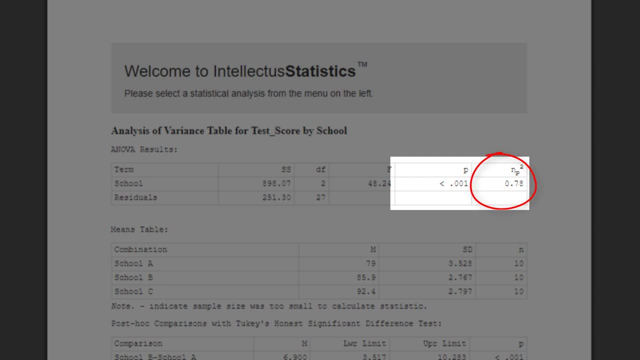 number between 0 and 1, but it's not a probability. Instead, eta squared measures the proportion of variance accounted for by the independent variables. That also means that higher is better. In this case, the eta squared is really high. It tells us that over 70% of the variance 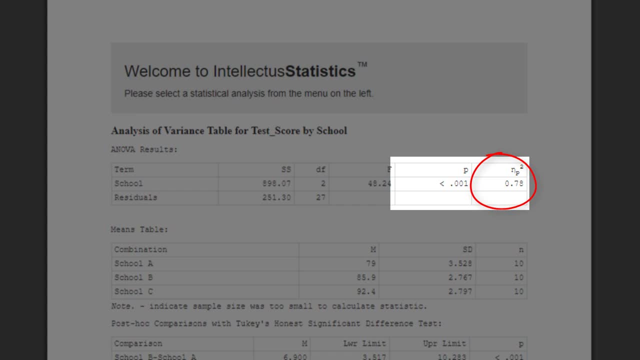 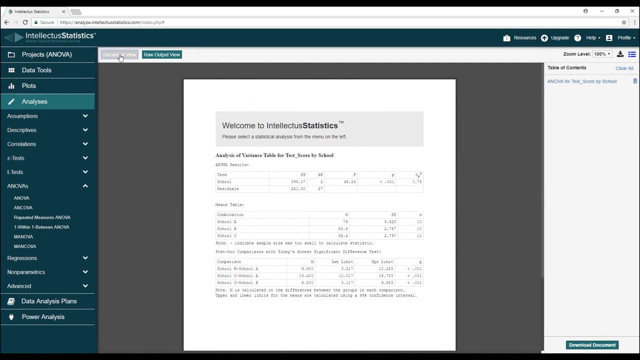 is explainable by the school the students attend. This reinforces the statistical significance. Okay, we're almost done. The last thing we need to do is look at the plots I mentioned earlier to see. if the assumptions were met, We'll switch over to the document view to look at the 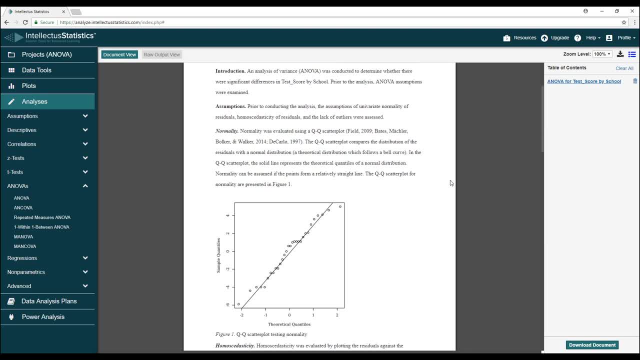 assumptions. Most of statistics isn't perfect. There are many things that are only approximations or that only work under certain conditions, and the ANOVA is no different. For one, it only works when the process that produced the data is normally distributed with equal variance across groups. 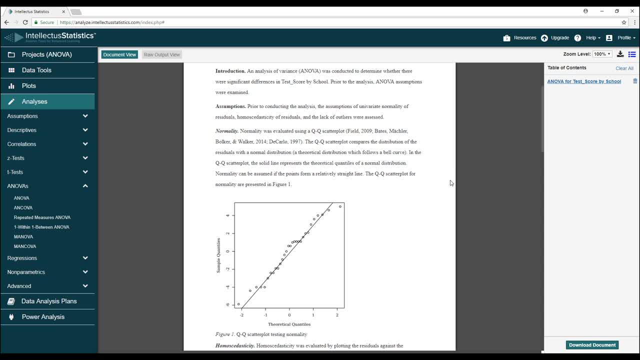 The data also have to be independent. These are called assumptions, because we assume these conditions are true when performing the calculations. That means that all of the results we calculated only apply if those conditions really are true. We have to look at some special values, called residuals, to decide whether the 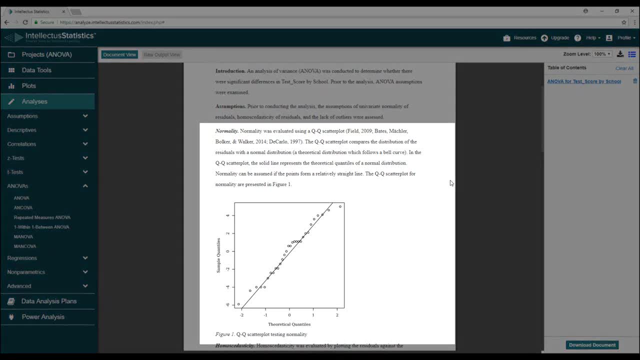 assumptions are met or not. Let's look at the normality assumptions first. There are many methods for this, but probably the most common is to just assess the assumption visually. This is called a normal quantile quantile or Q- Q plot plot. This plot compares our residuals with a normal distribution. What we want here is: 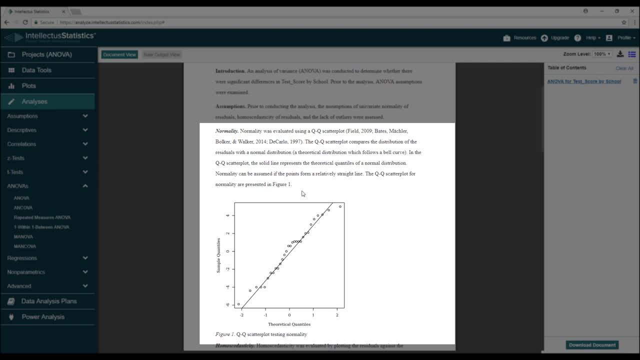 for the points to follow the line. There will always be some deviations, but as long as they're small and there's no pattern or curvature, we can say the normality assumption is met. Here you can see examples of normal and non-normal distributions, In this case the sample size. 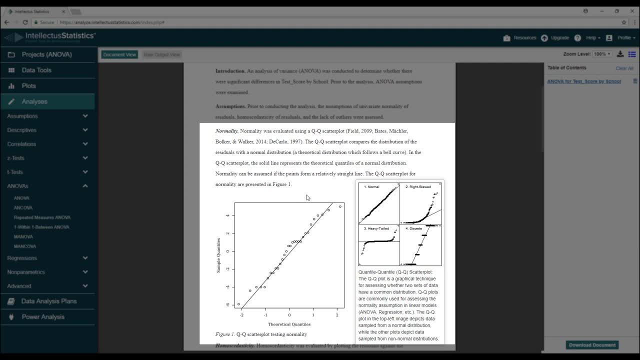 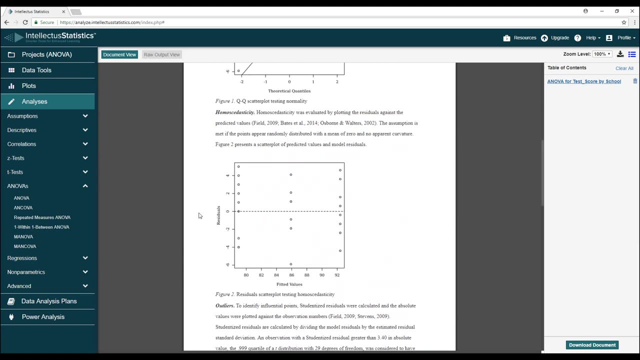 is small, so there are a few deviations, but they appear to follow the line well enough. so we'll say the normality assumption is met. The next plot uses the same residuals as the Q-Q plot, but plots them against the group means on the x-axis. What we want here is: 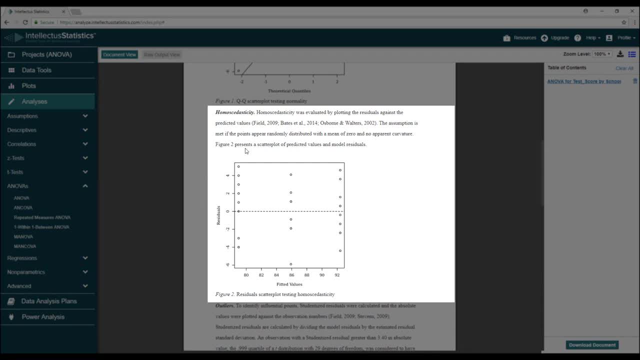 to see each set of points centered at zero and to have about the same variance. That means each set of these points should look about the same, with similar minimum and maximum. It looks like that's the case here, so the equal variance assumption is also met Sometimes. 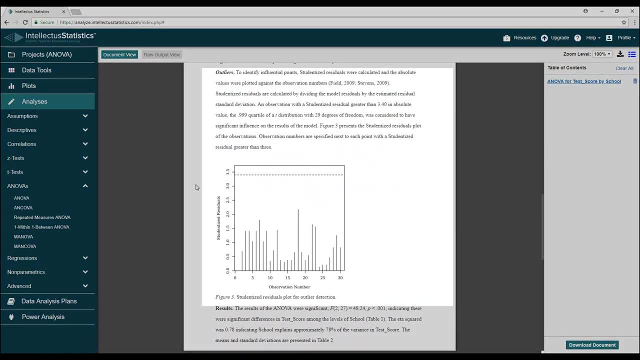 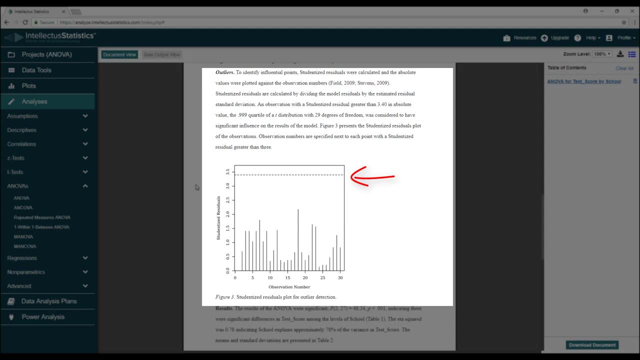 it can be hard to identify outliers using the Q-Q plot alone, so an additional plot called the studentized residual plot can be used. Any points which are above the line indicate observations which could be designated outliers. The most critical assumption is that the data need to be sampled randomly and independently.